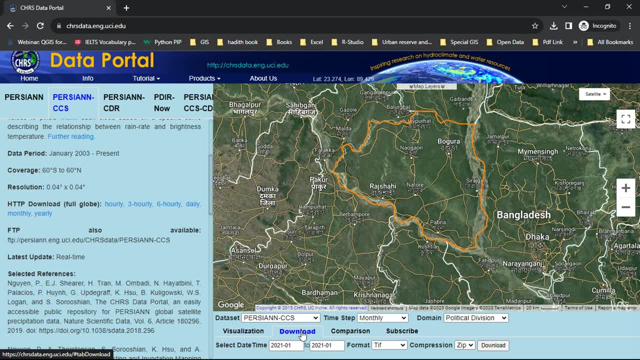 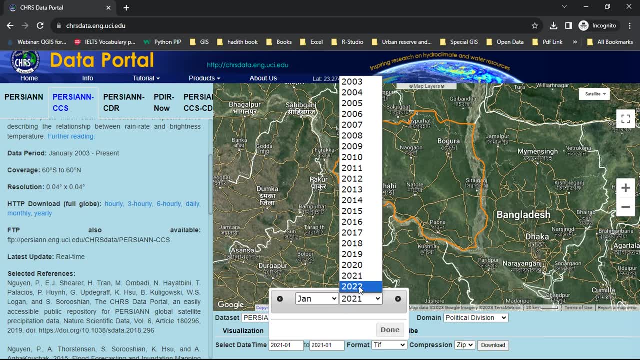 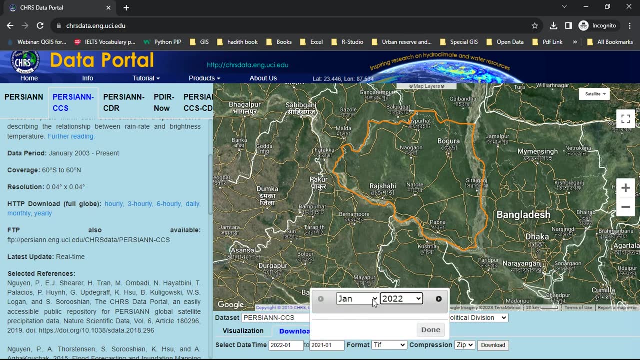 area it, it will be highlighted. now select this option- download- and then select the date. and let's say, i want to download the data of 2022, of january, okay, to 2022, june. then click on done and in the format section you can choose any of these either: r, grid, tif, net, cdf. i want to download it as tip format, so i am. 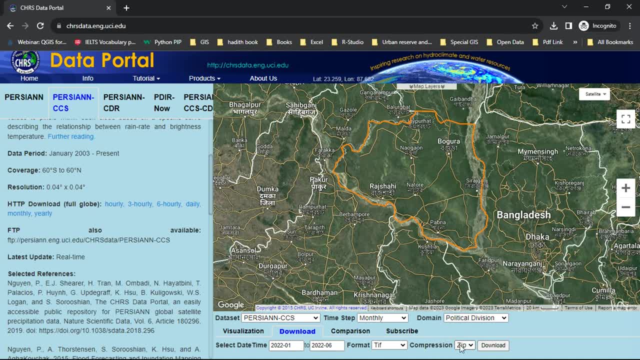 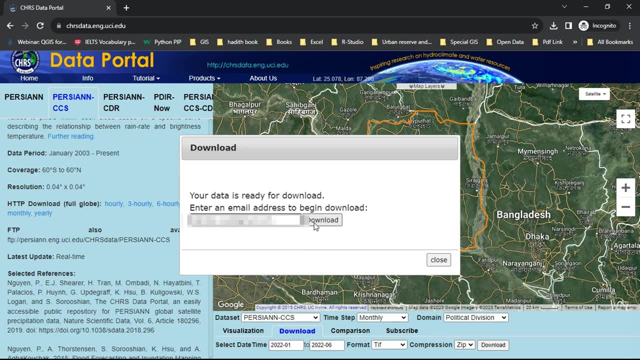 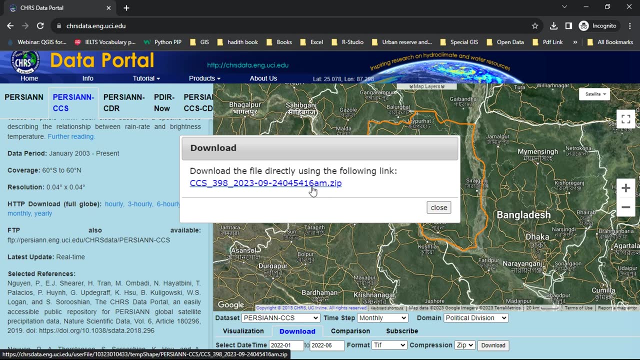 selecting this one and then in the compression i will select this one. zip, then click on download. now you have to provide your email address. after providing your email address, click on download now you will see the download link of the data. click on this link to download the data. 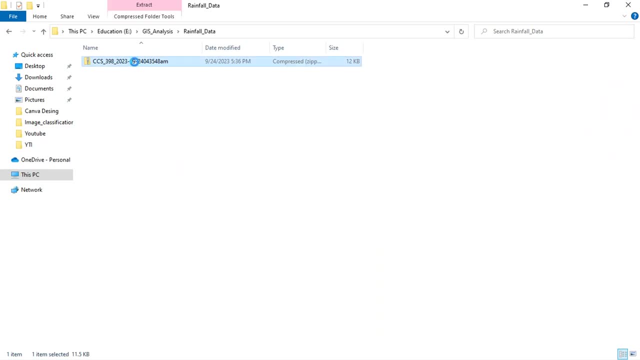 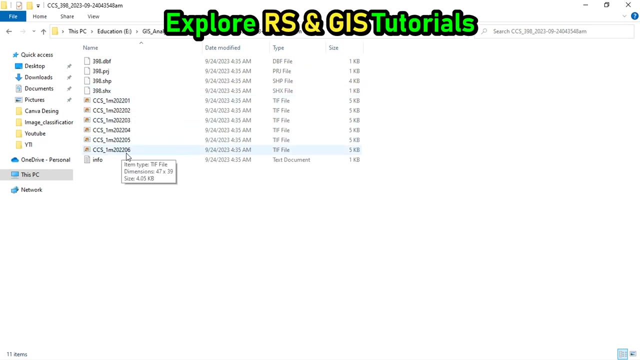 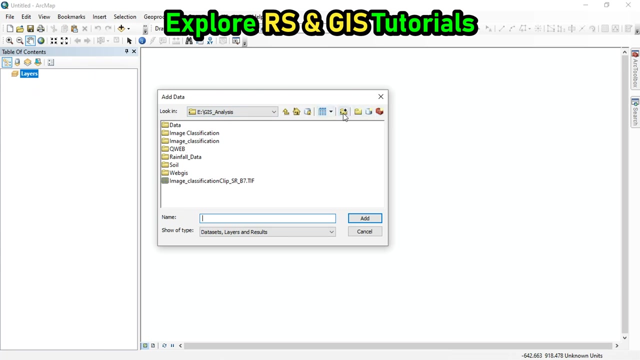 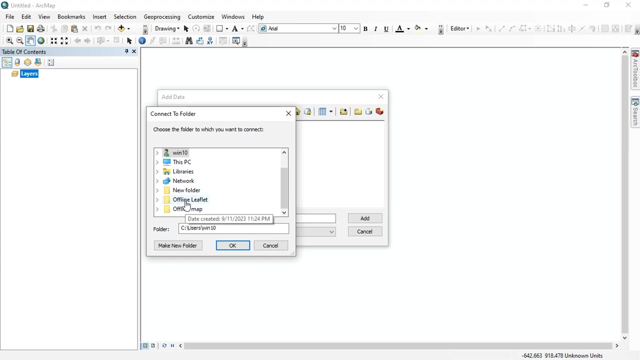 so here is my data that i have downloaded recently. now i'm going to unzip this. here is my data from 2022: january to 2022: zoom. let's open this data now. if your folder is not connected, you can connect your folder by clicking on this. then select the folder where you store your data. in my case, i already connected. 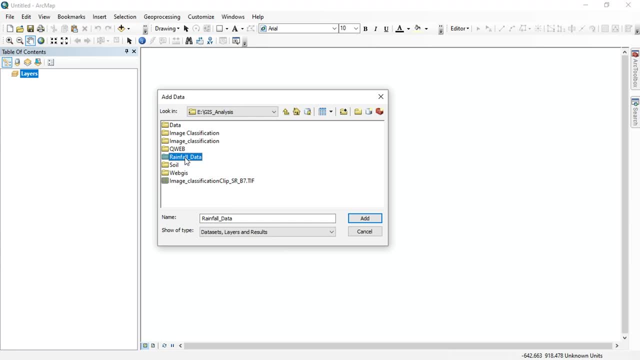 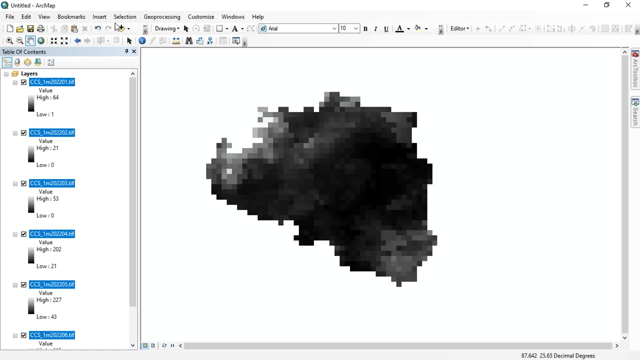 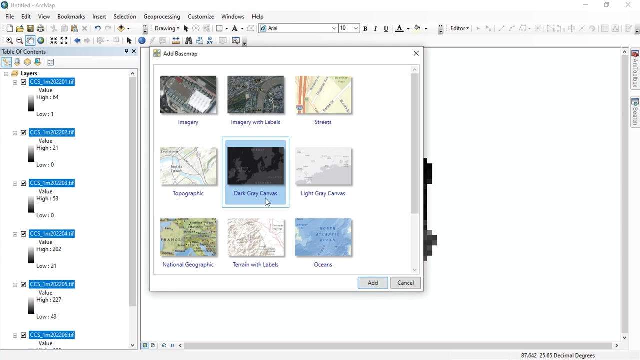 that folder. here is one: the rainfall data and these are all my data. click on add to add all that raster data. click on ok, you can also add base map, if you want, by clicking on add base map. i want to add this one dark gray canvas. then click on that. this one shows some error. 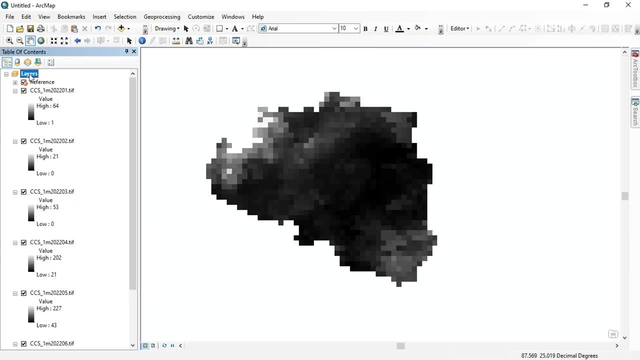 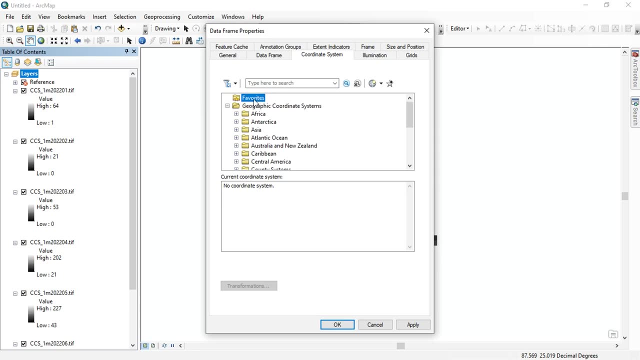 you have to define the coordinate system. you know you have to define the coordinate system. you know that you do that. click on layer, then go to properties and from here select this one coordinate system, then select this one geographic coordinate system and this one world. wgs 1984. 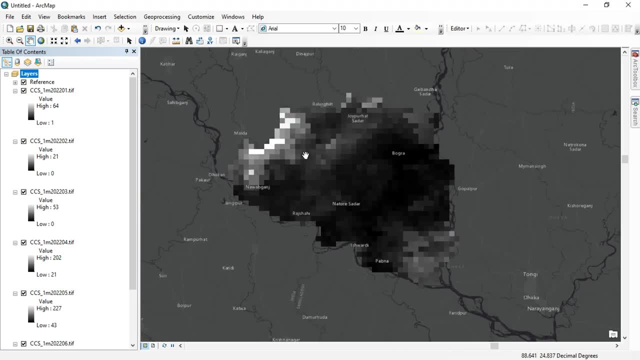 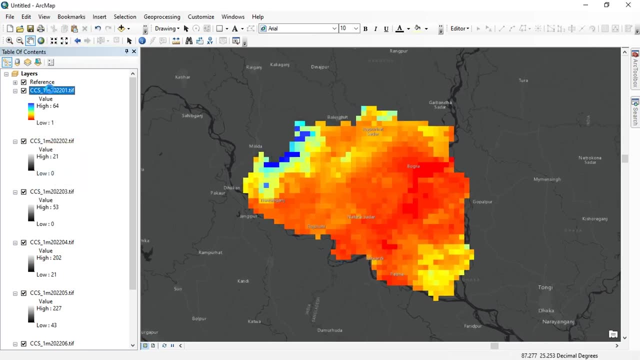 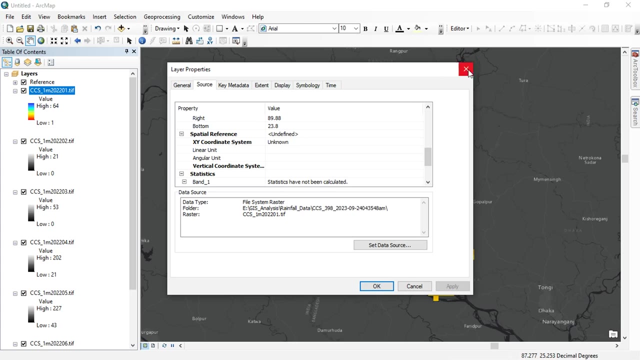 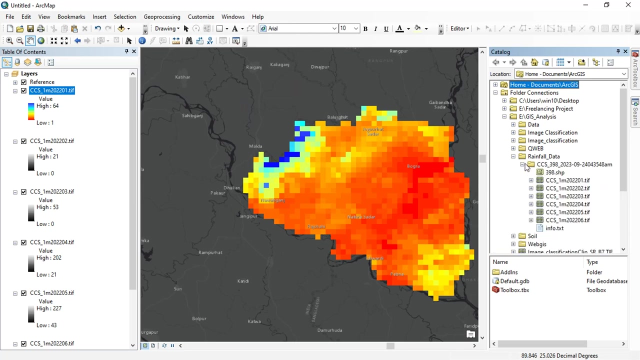 then click on apply. you can also change the symbology of these by clicking on this tab. then select the symbology, click on ok, here it is. let's check the coordinate system by going to the properties. special reference system is undefined. you can easily define these from catalog to the folder where you store your data. then select this one, go to properties.